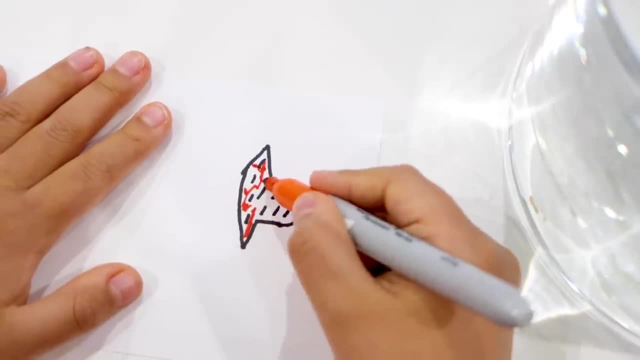 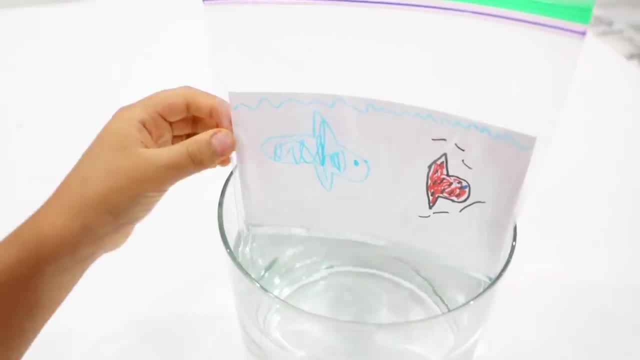 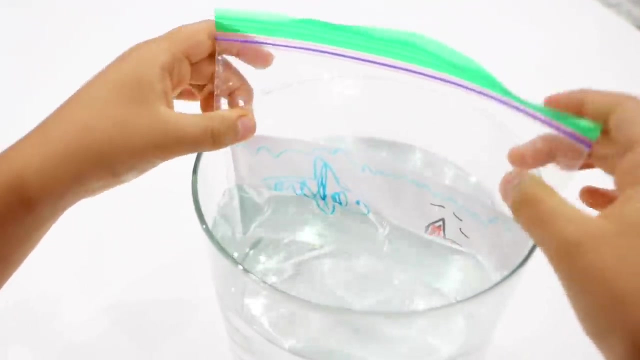 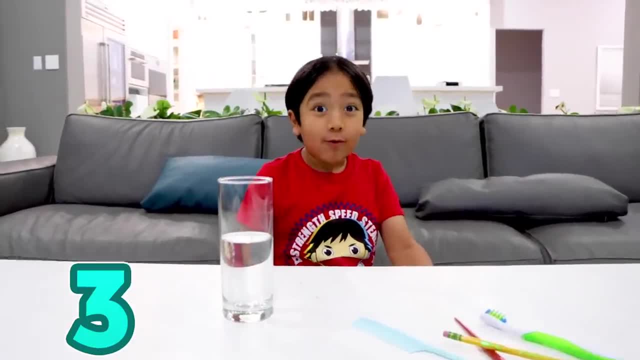 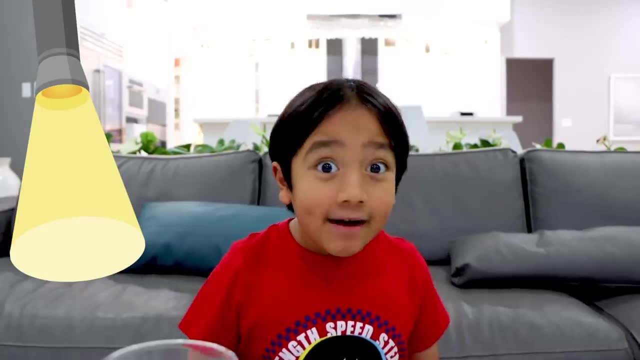 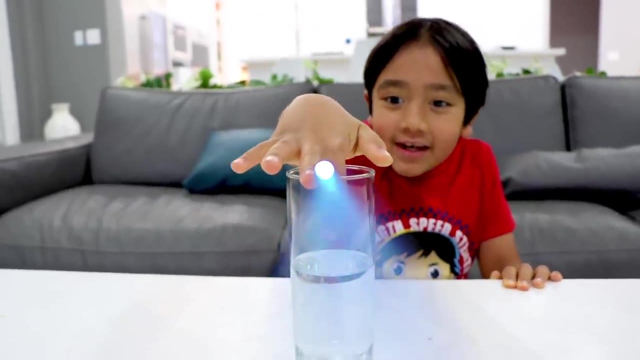 Hey guys, today I'm going to show you three really cool water refraction tricks. What is refraction, you ask? Well, refraction is the bending of light while it passes through a new medium. So the light is going through the air and then suddenly it goes into the water. All you need 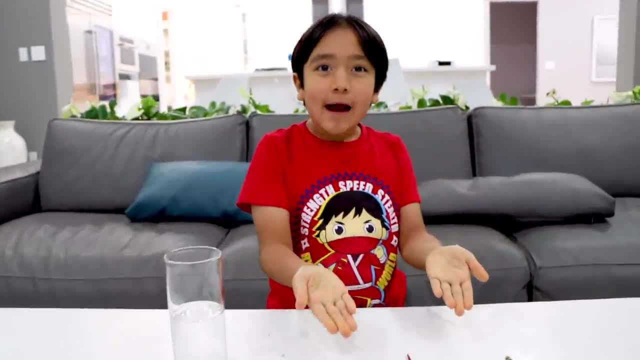 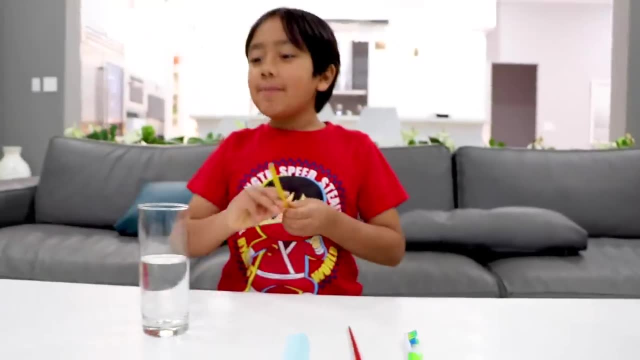 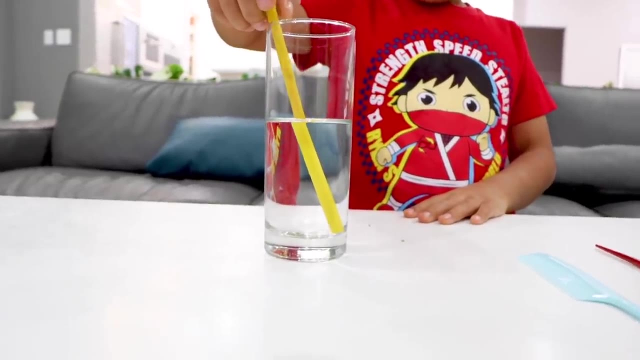 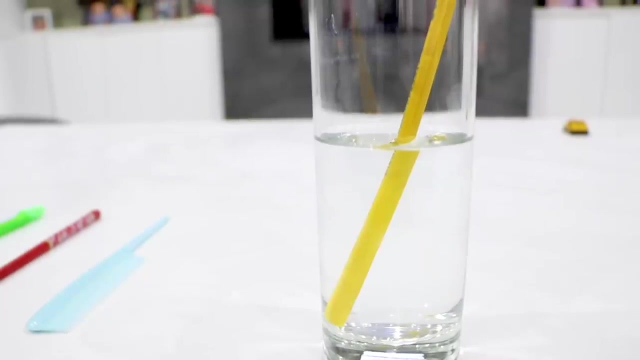 is a glass of water and some objects around the house. It could be anything, but these are the objects I chose First. let's try it with a pencil. So see, it's going here, and then it bends And it looks a lot bigger too. Guys, did you see how the water makes it look like the pencil is bent? 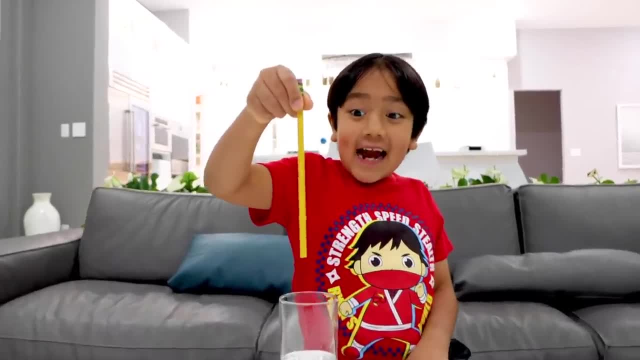 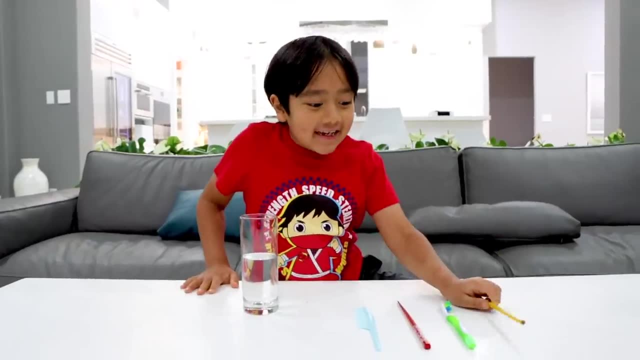 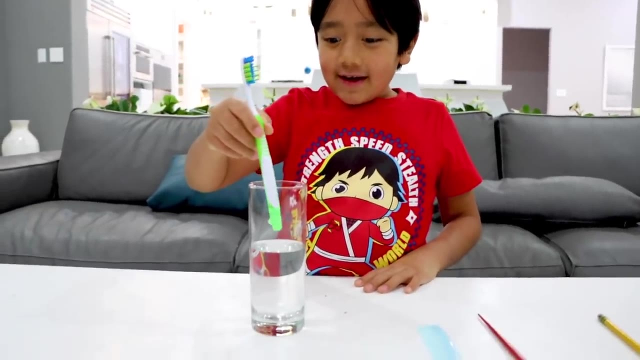 That's really cool, right? Well, my pencil isn't actually bent, It's just refraction Bending of light. Okay, let's test out other objects to see if it works too. Let's test out this toothbrush, Okay. 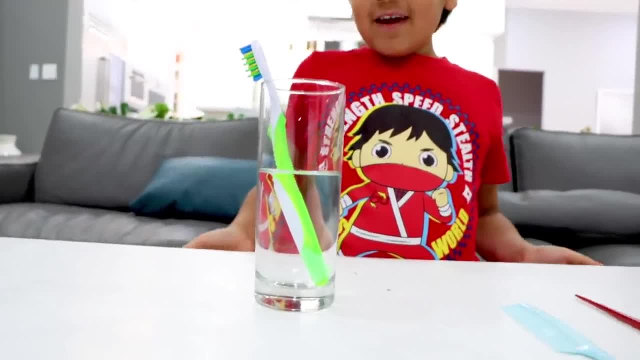 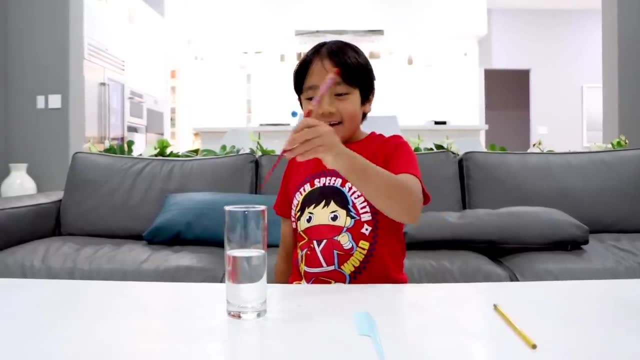 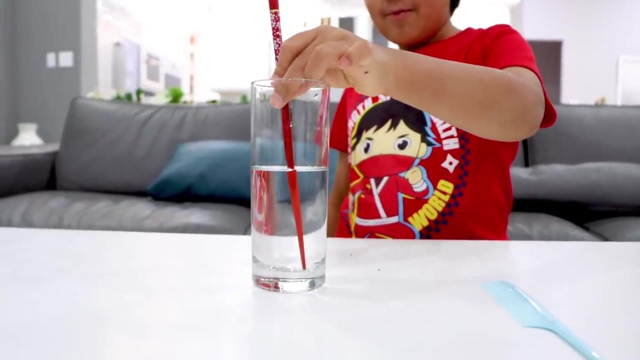 Whoa, it looks so cool, It's so much bigger And it bended too. That's so cool. But what about chopstick? Okay, here's a small part. It's getting bigger, bigger, bigger, Boom. Whoa, that's super big. 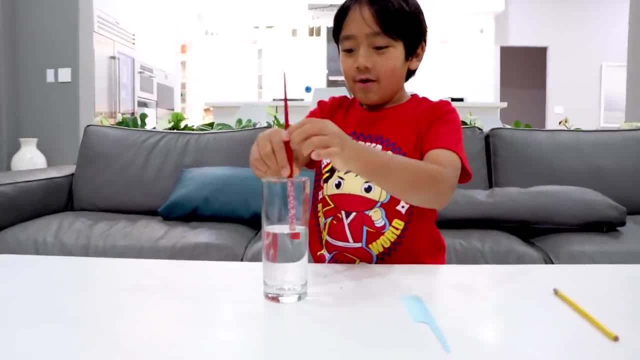 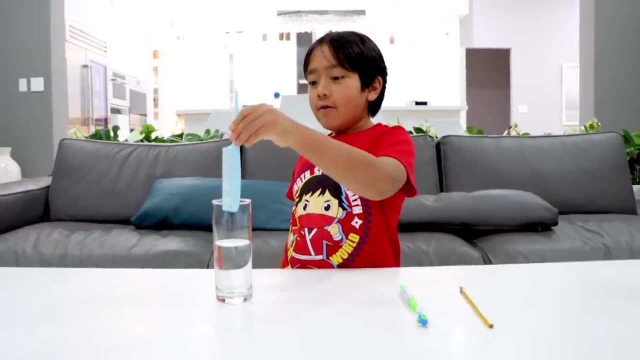 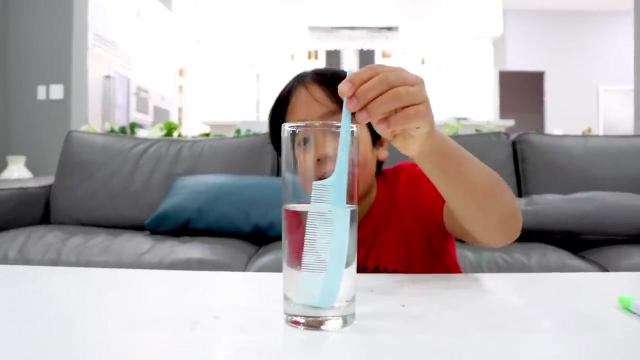 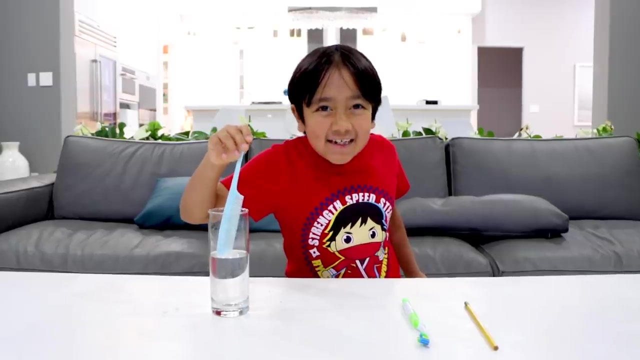 Let's try the other part. that's already big. Whoa, it's bending, and it's super big. Okay, what about this comb? Whoa, Whoa, that's so cool, It's bending. So why did it look like the object bent under the water? Because of refraction On to number two. 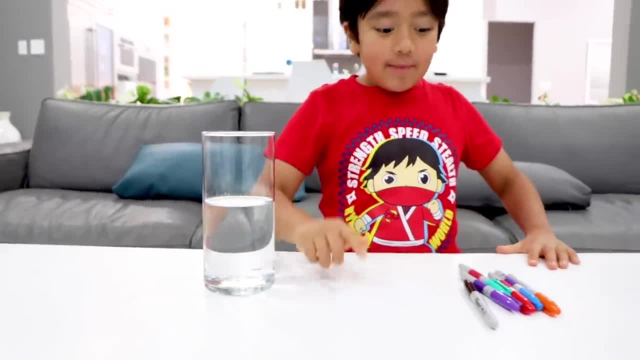 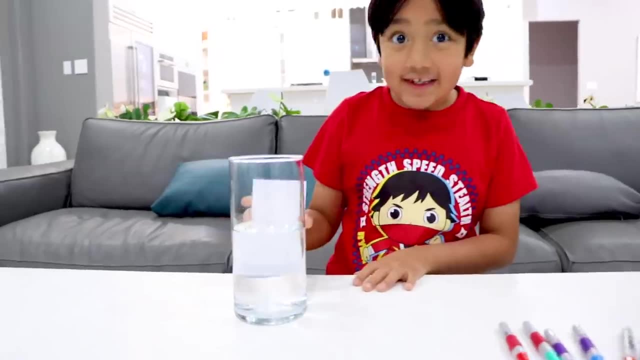 So for the next trick, you're going to need a glass of water, paper and some markers. Okay, guys, so for this one, I'm going to draw it and put it on the other side and something cool will happen. I'm going to draw an arrow with multiple colors. So first red. 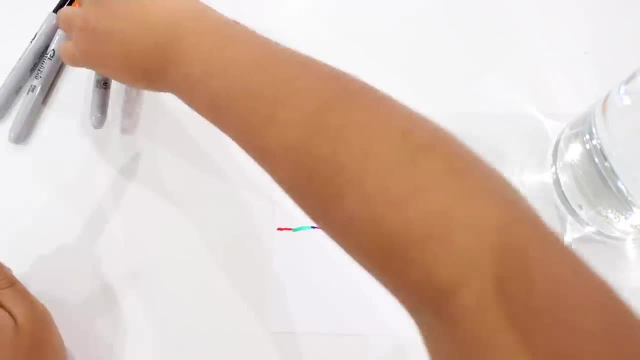 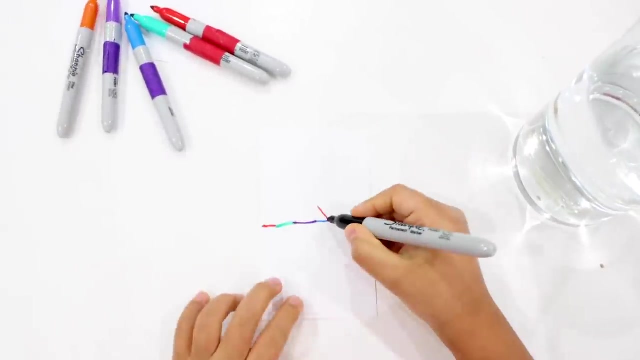 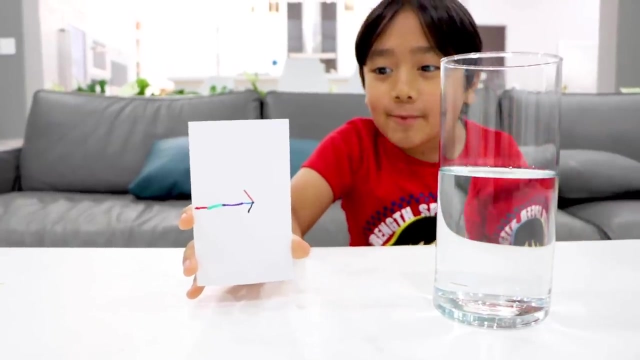 and then teal, purple, and then blue, and then orange and blue. So you guys see that this is an arrow. Well, look at what direction it's pointing at. It's pointing out that way When you put it behind the water. 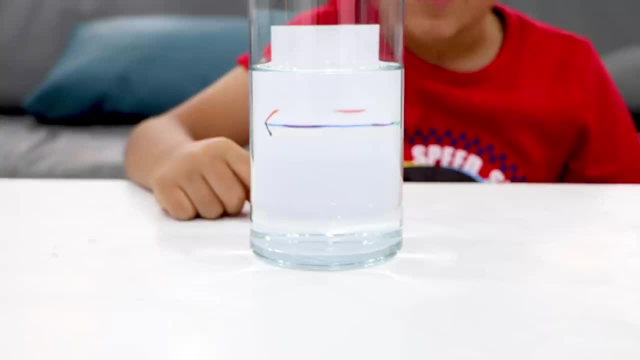 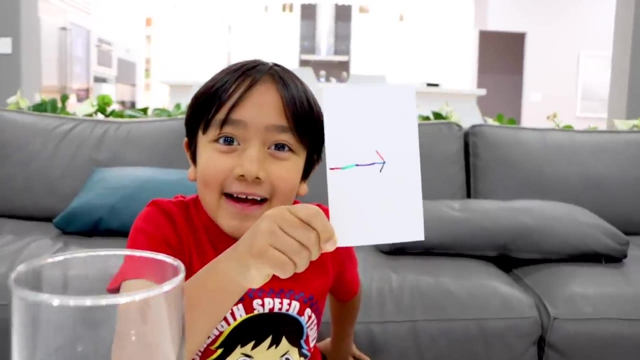 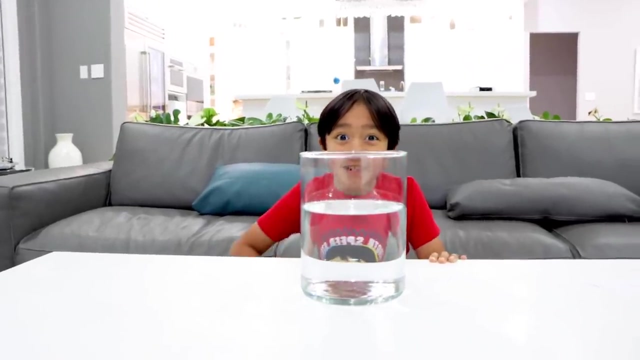 it points the other direction, So it's reversed, Isn't it cool? Well, that's just refraction. Still going the same way. now, Before I show you refraction trick number three, here's a bonus one. Look what happens to my face. 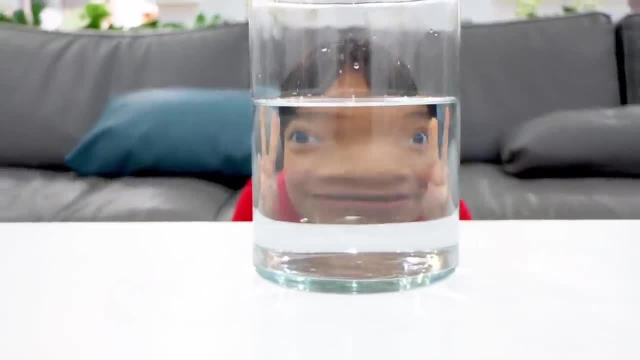 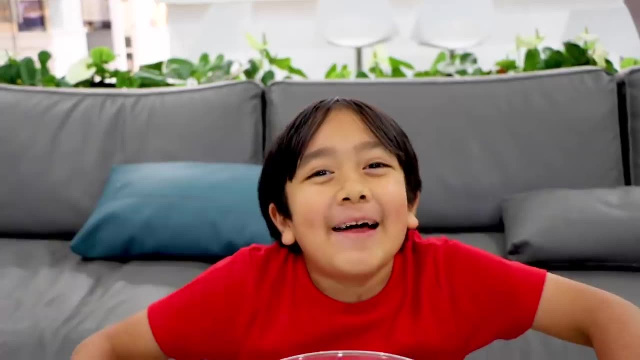 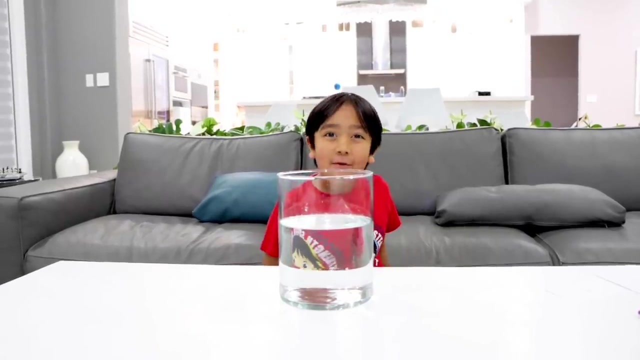 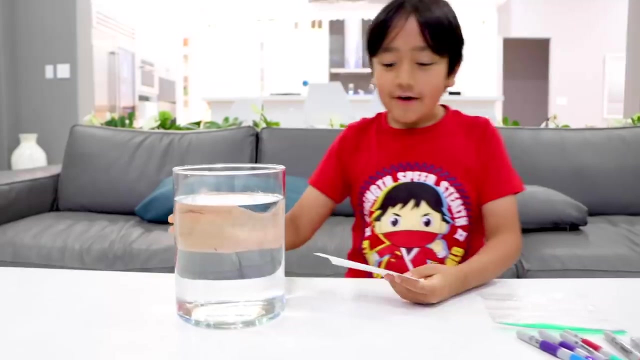 Hi, What's up? Oh yeah, peace. Oh, Now I'm all better again. See, Now my face is normal. It's just refraction. Now for trick number three. Okay, so for number three you need obviously a container of water, some paper and a Ziploc bag. 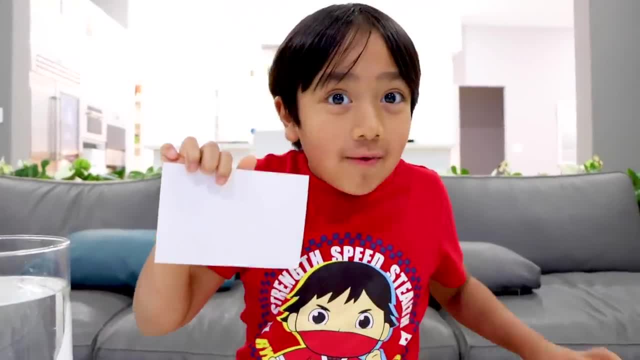 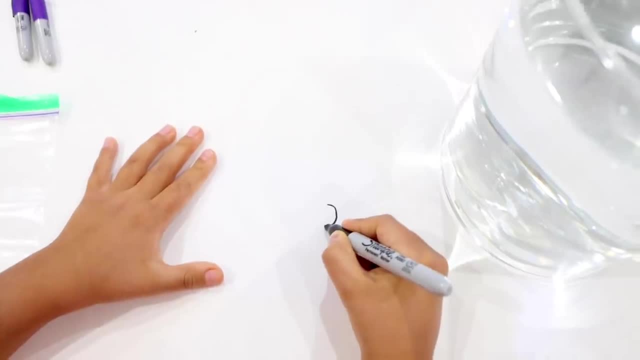 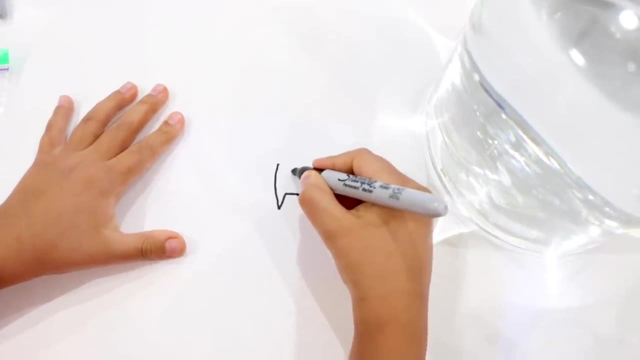 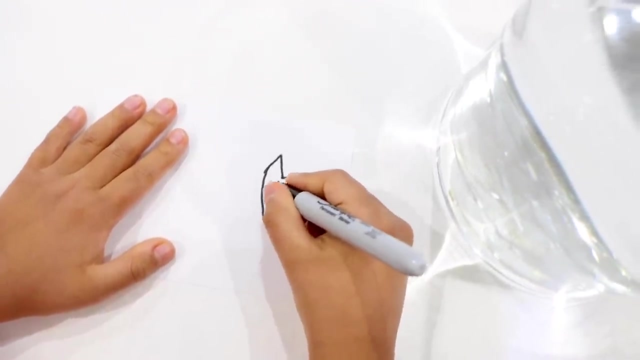 First step: draw something on here. Draw whatever you want to disappear. Okay, I'm gonna draw a fish Like this, And then a little bit more here, Bam. And then here, here, here, Bam, Perfect fish. Okay, I'm gonna draw its scales. 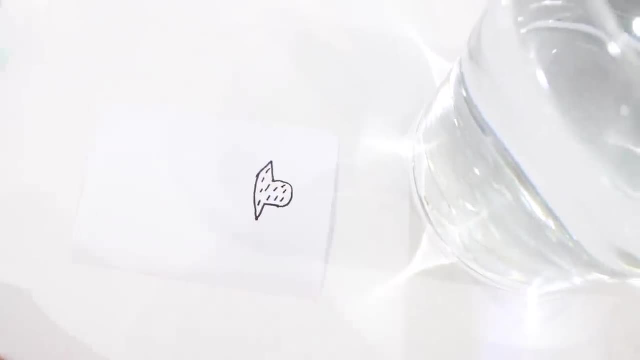 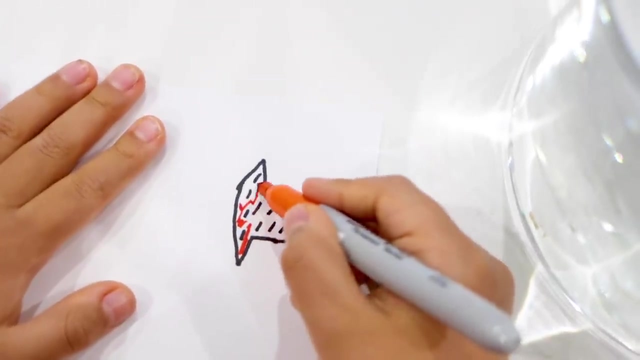 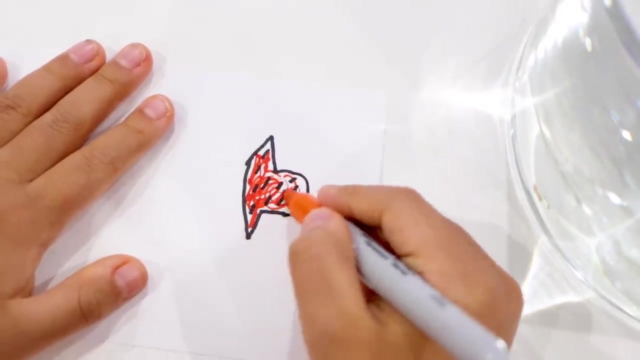 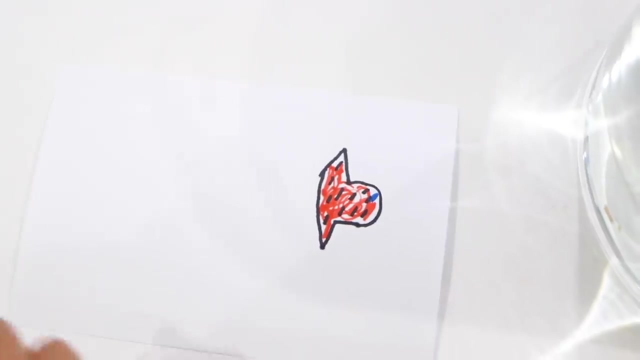 Like this, that this: Okay, there you go. Then I'm gonna draw it in The perfect, definitely drawed-in fish, Okay, and then I'll put an eye on this side And then I'll put some running away, some running away dashes. 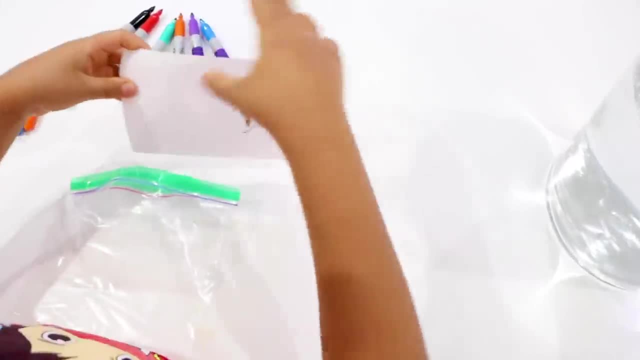 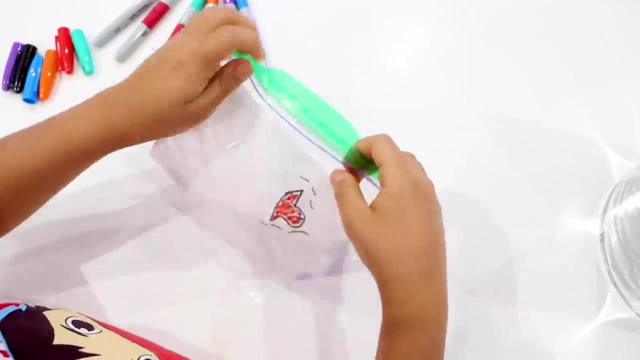 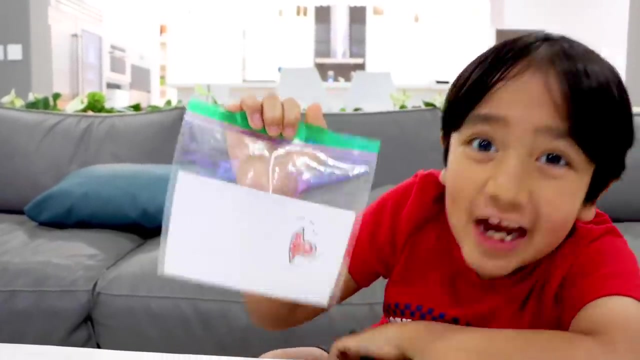 Then you're gonna put it in a Ziploc bag, Okay, like this. Okay, now I'm done with my fish and I put it in. So now I'm gonna draw a shark chasing the fish. Draw a super good shark, like this: